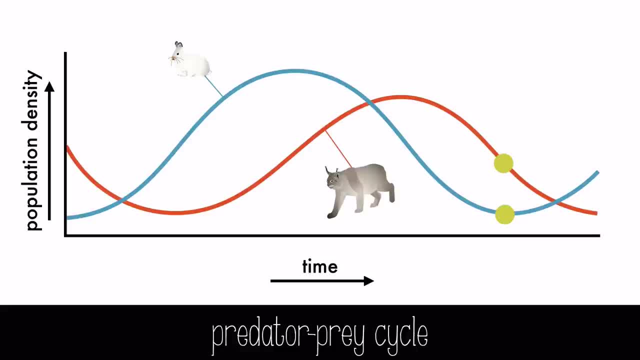 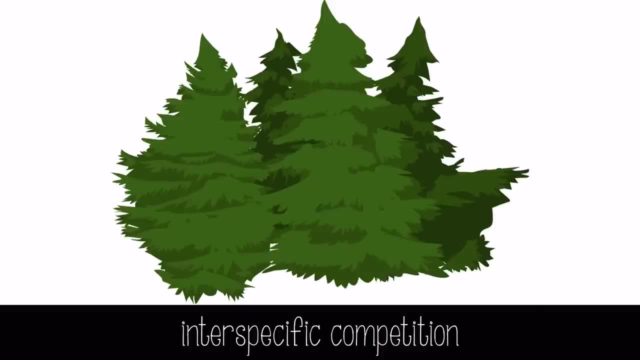 once more, the predators will also increase their population. It's a cyclic pattern. Interspecific competition is the type of interaction in which two or more species use the same limited resource. For example, two species of birds in the same habitat might try to. 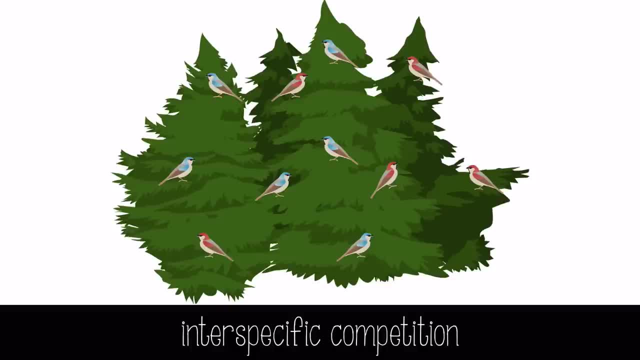 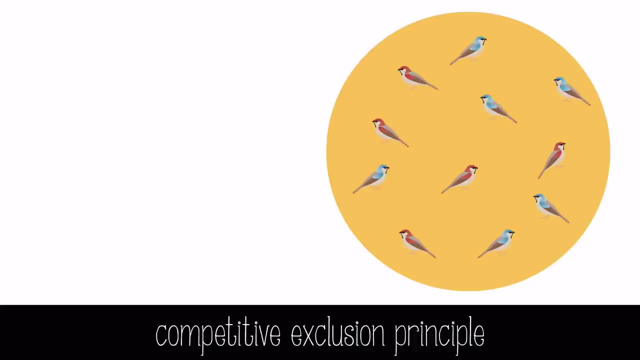 occupy the same niche, eating from a tree, And both lions and hyenas compete for prey, such as zebras, and many plant species compete for soil or sunlight. Some species may be better at getting their resources than others. The competitive exclusion principle describes situations in which one species is eliminated from a community because of competition for 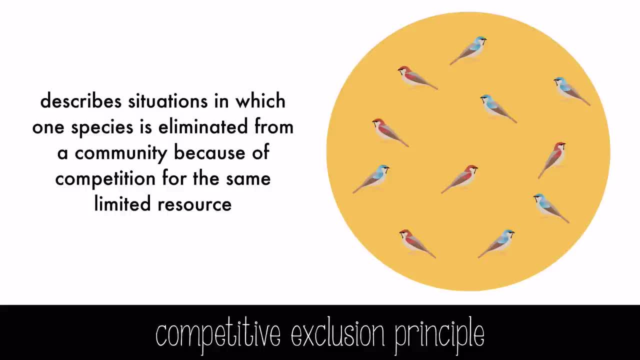 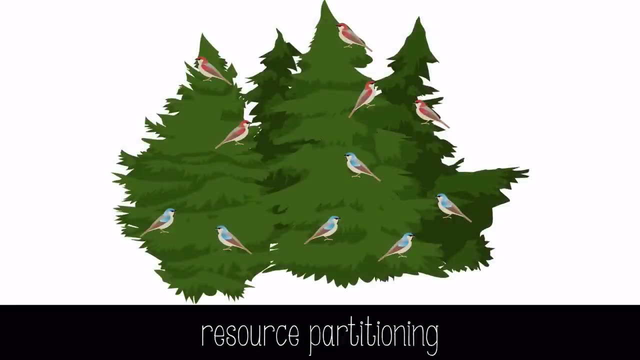 the same limited resource. Often, one species is more efficient than another at getting their resources. In order to avoid too much interspecific competition, the birds in this habitat may choose to do something else. resource partitioning When similar species coexist. each species may avoid competition with others by using a specific part of an available resource. 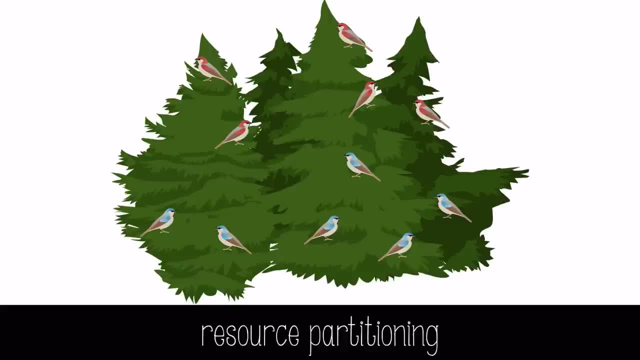 This is called resource partitioning. In the case of these birds, they will claim different parts of the tree. The red birds will feed and live up at the top, and the blue birds will feed and live at the bottom. By staying out of each other's way, they can both survive in the same habitat. 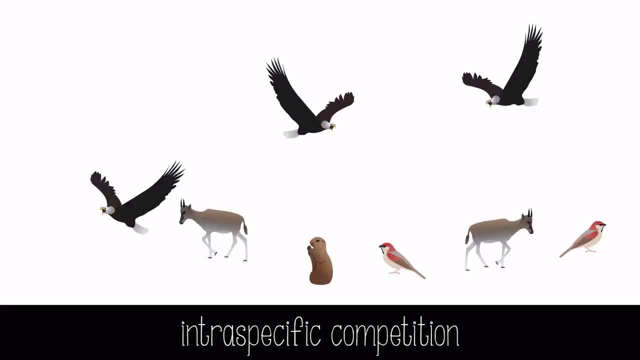 Intraspecific competition is the type of interaction in which two or more individuals of the same species use the same limited resource, like food or water or mates. For example, two trees of the same species growing close together will compete for light water and nutrients. 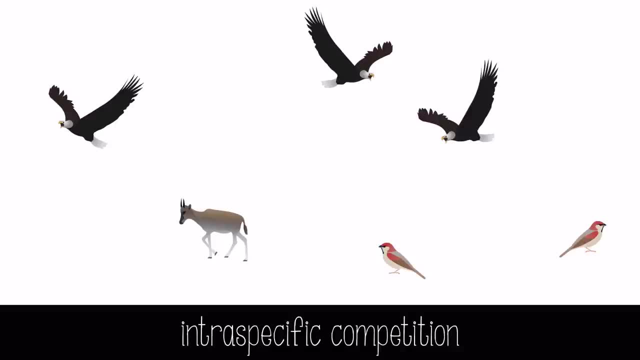 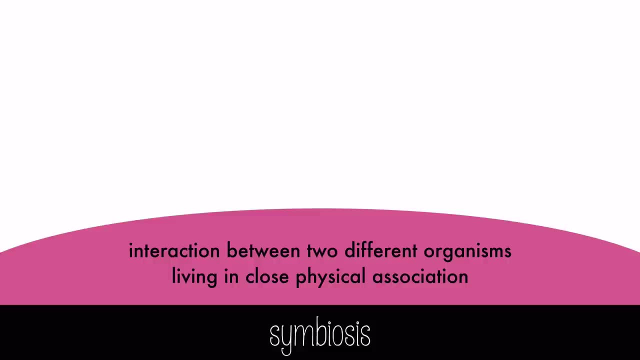 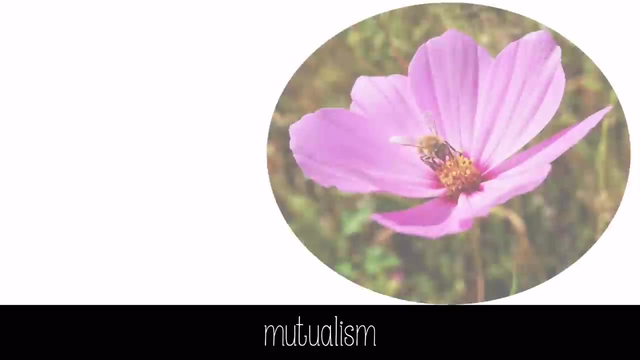 in the soil, And these equals are all competing for their different food types. Symbiosis is an interaction between two different organisms living in close physical association. There are three types of symbiosis: Mutualism, commensalism and parasitism. Mutualism is: 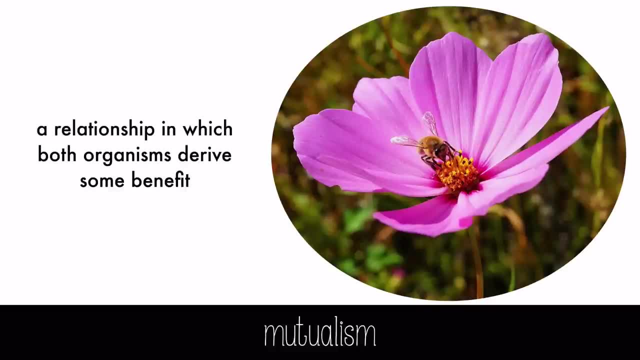 a relationship in which both organisms derive some benefit. An example is flowers and their pollinators. like bees, Flowers provide food and the pollinators carry pollen to other flowers. It's a mutual benefit to both species. In commensalism, one organism benefits the.